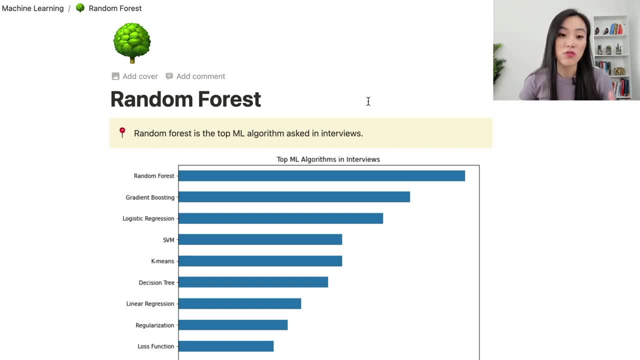 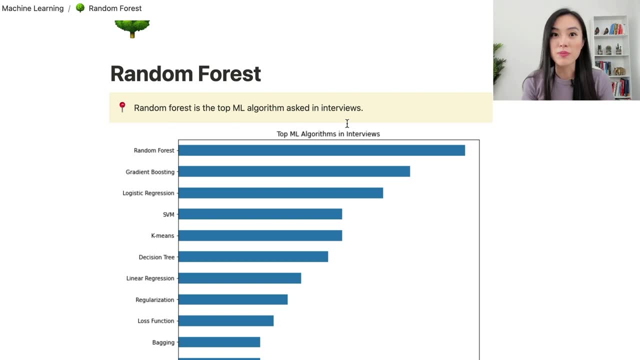 Hey guys, in this lesson let's talk about random forest. Random forest is the top machine learning algorithm asked in interviews And in this video we will dive deep into random forest. After watching this video, you will be able. majority of interview questions related to random. 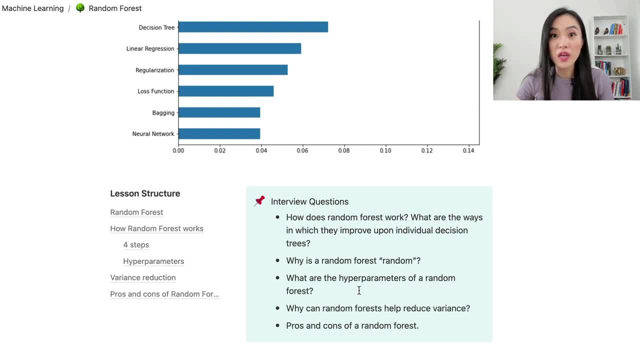 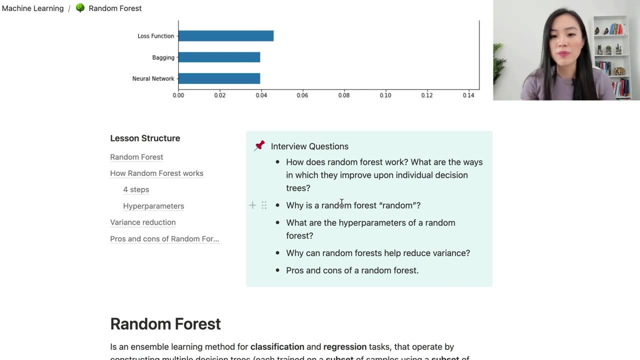 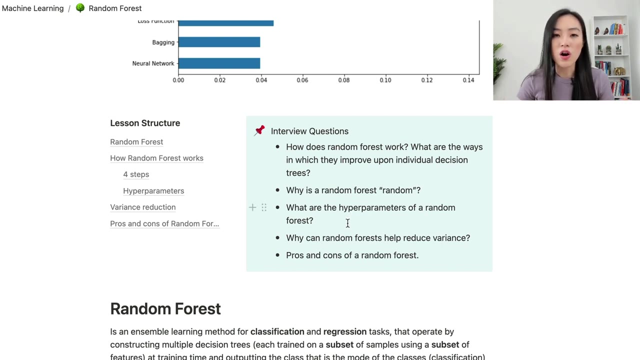 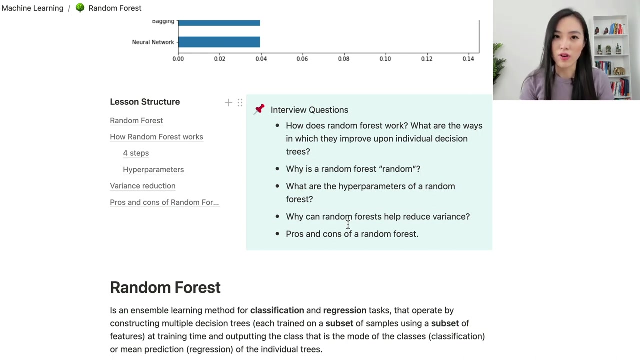 forest. Let's get started with looking at some interview questions. How does random forest work? What are the ways in which they improve upon individual decision trees? Why is a random forest random? What are the hyper parameters of a random forest? Why can random forest help reduce variance? Pros and cons of a random forest. 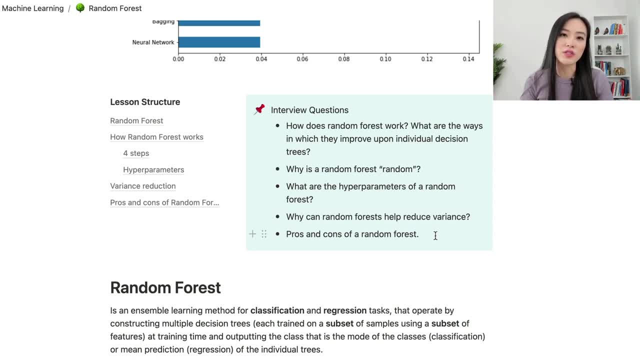 These are all fundamental questions related to random forest And we will go over all of them in this video. Specifically, we will look at what is a random forest. How does it work? There are four steps In the algorithm. we will go over all of them one by one. And what are the hyper parameters? 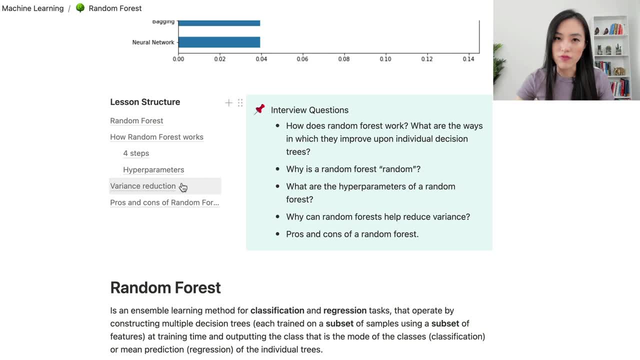 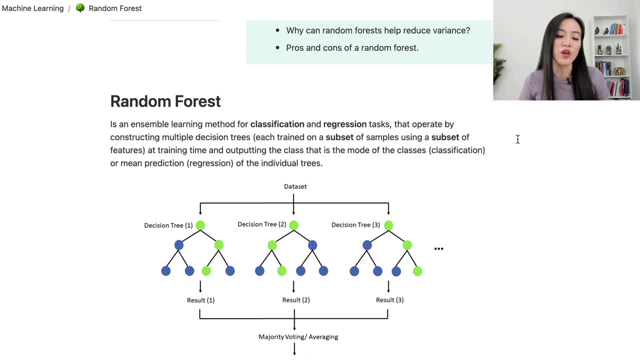 of a random forest, How does random forest reduce variance? And finally, we will summarize the pros and cons of random forest. Okay, let's start with reviewing what is a random forest algorithm. A random forest is an ensemble learning method for both classification and regression tasks. 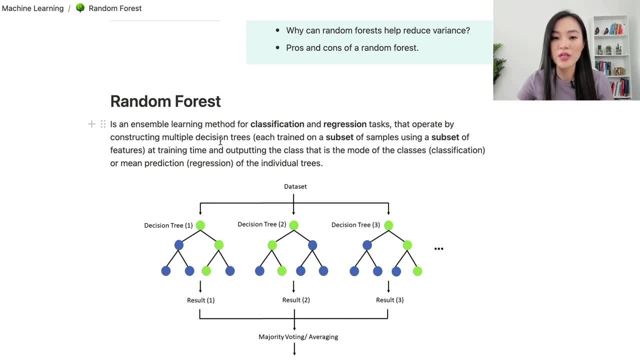 It operates by constructing multiple decision trees. Each tree is trained on a subset of samples using a subset of features. We will talk about the benefit of doing this later on. So once it constructs multiple decision trees at training time it outputs the class, that is, the. 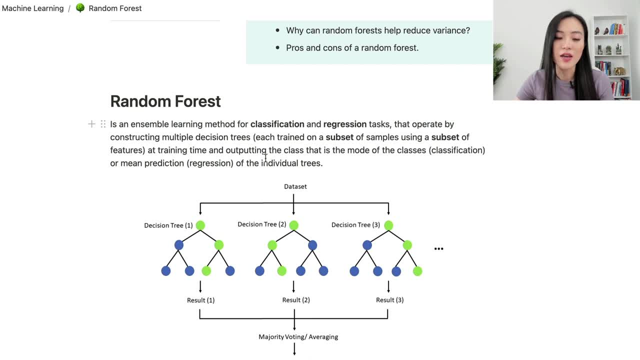 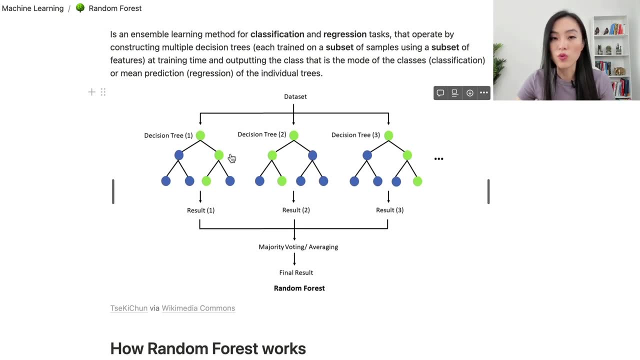 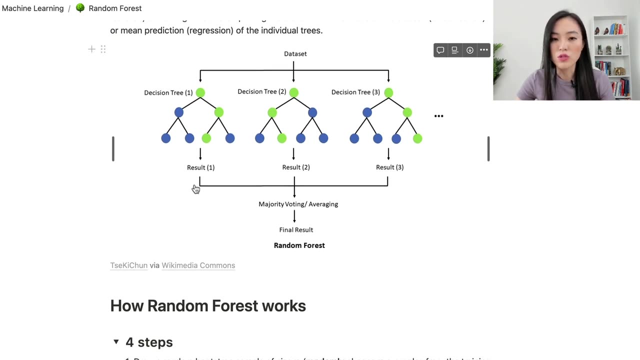 mode of the classes for classification tasks or mean prediction for regression tasks of the individual trees. Here is a diagram showing how it works. So in this case there are three decision trees: one, two and three. The random forest algorithm looks at the results of all these trees and then take majority voting or averaging. 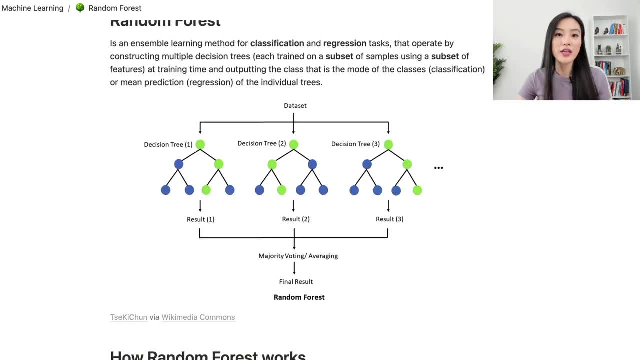 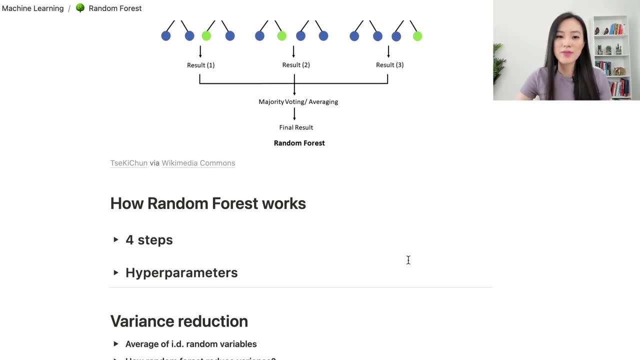 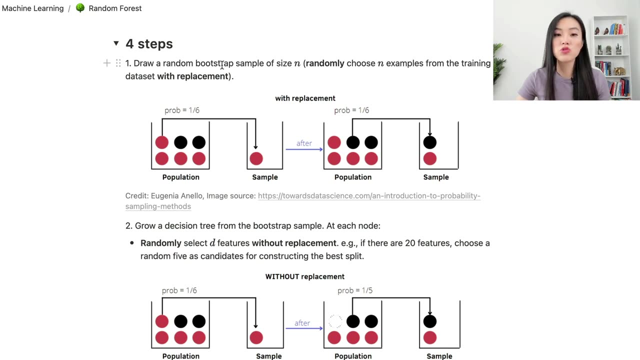 and then output the final result At a high level. that's how a random forest works. Now let's look at the details and understand how it works step by step. There are four steps in the algorithm to construct a random forest. We first draw a random bootstrap sample of size n. We randomly choose n examples from the training. 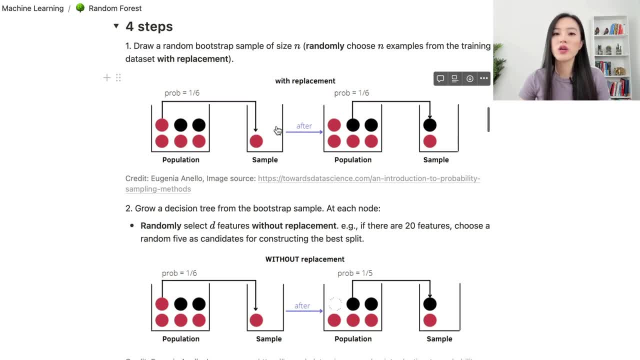 dataset with replacement. Here is the diagram showing with replacement. So when we draw a sample from a population, we put it back before we draw another sample. So essentially it means that one training example may appear multiple times in the bootstrap sample. The second step is that 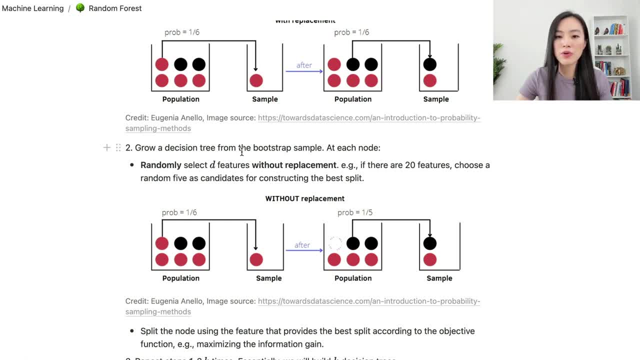 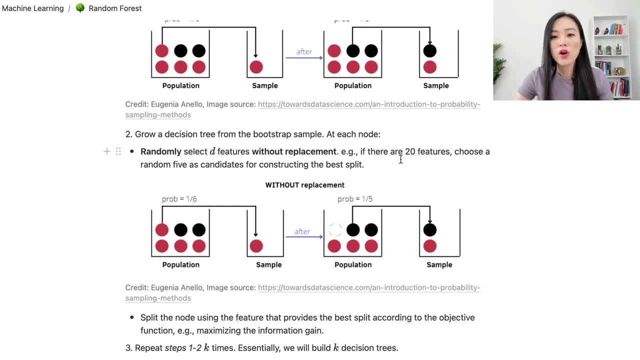 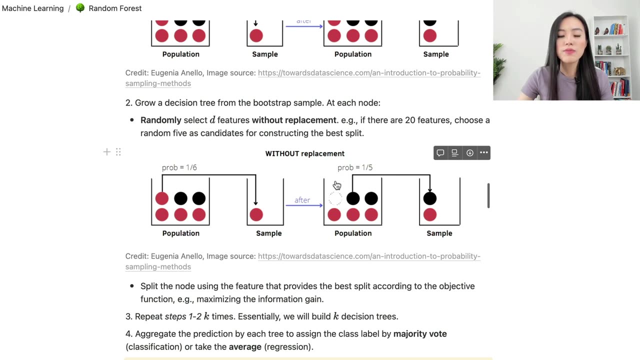 we grow a decision tree from the bootstrap sample. At each node we randomly select the features without replacement. For example, if there are 20 features, we choose a random 5 as candidates for constructing the best split. So here is the diagram showing, without replacement, When we draw. 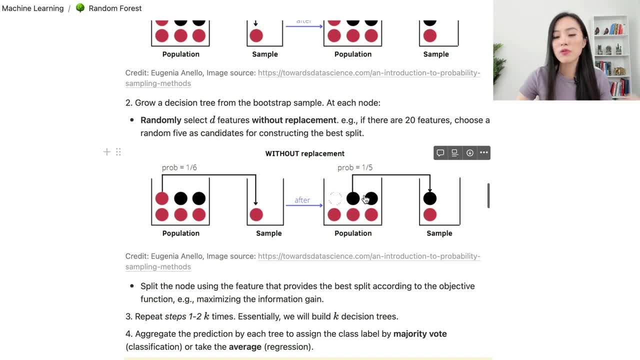 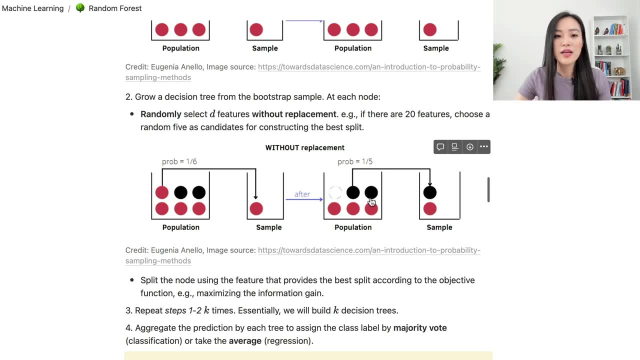 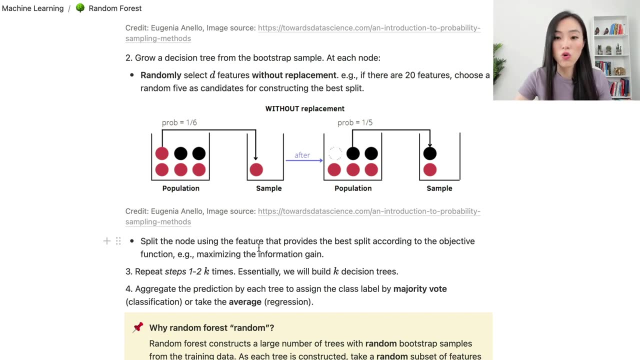 a sample from a population, we do not put it back before drawing another sample, So there is no duplication in the sample from the population. Once we select these D features, we split the node using the feature that provides the best split According to the objective function, for example, maximizing the information gain. 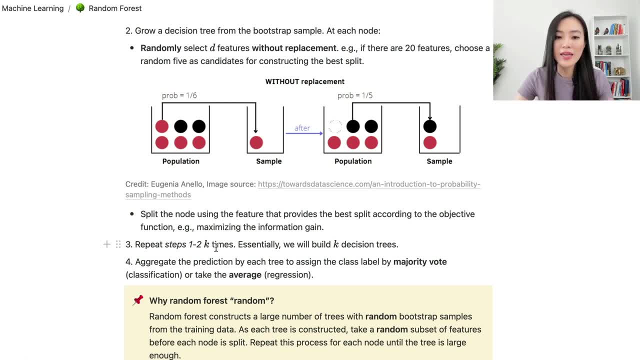 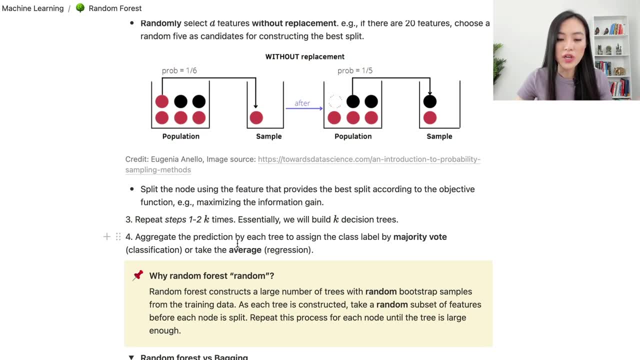 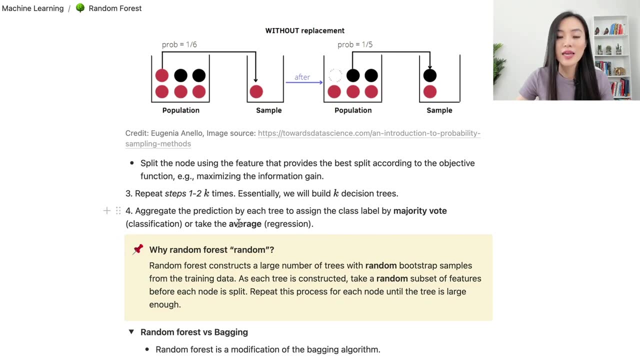 And then we repeat steps 1 to 2 k times. Essentially, we will build k decision trees. Finally, we aggregate the prediction by each tree to assign the class label, by majority vote for classification tasks or taking the average for regression tasks. 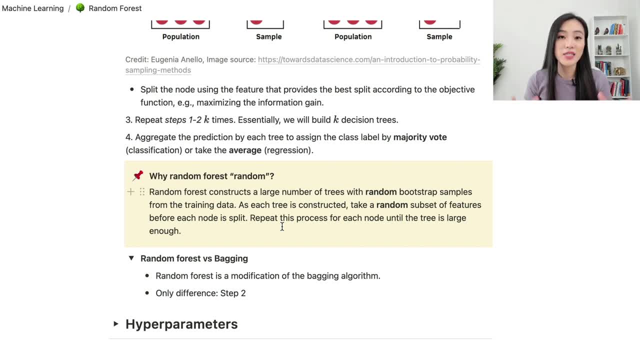 Once we understand this 4-step algorithm, it is easy for us to generate a routine for each class, for us to understand why. random forest, random Random forest constructs a large number of decision trees with random bootstrap samples from the training data As each tree is constructed. 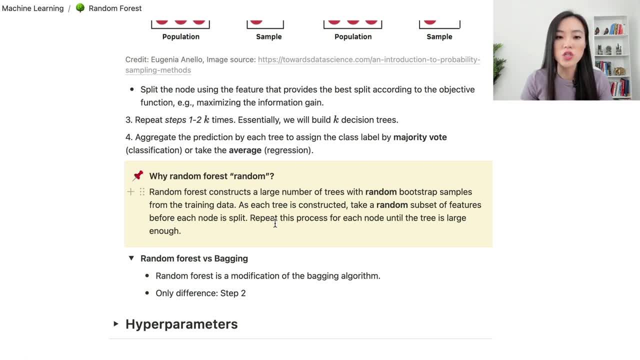 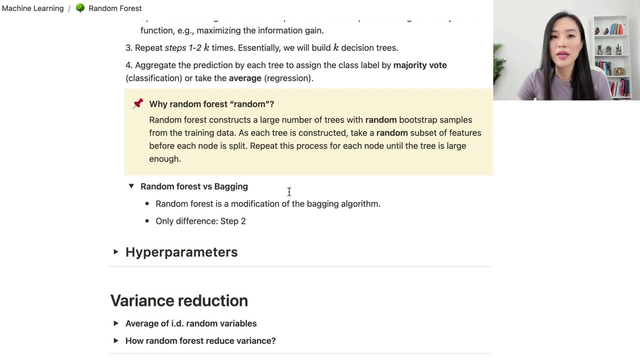 we take a random subset of features before each node is split. So, from step 1 and step 2, we introduce some randomness when constructing a random forest. That's why random forest is random. Now, for some of you who have heard about the bagging algorithm, bagging is an ensemble. 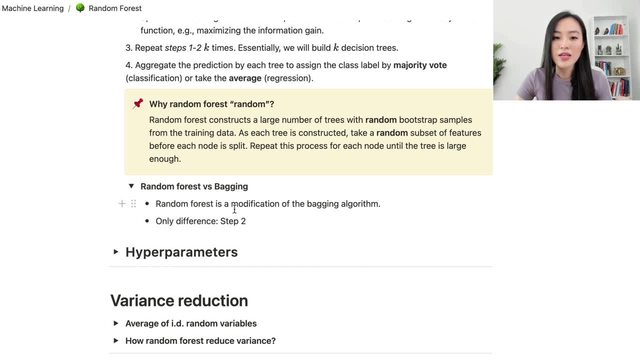 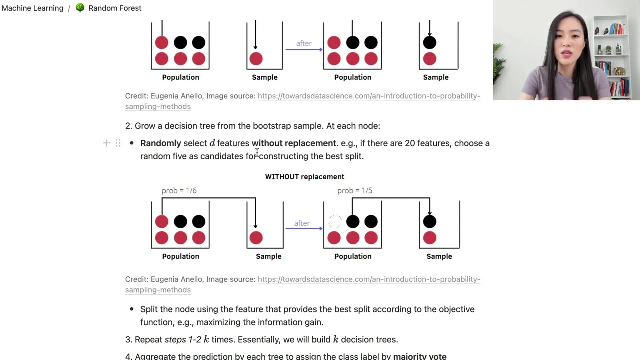 learning method. you may know that random forest is a modification of the bagging algorithm. The only difference between random forest and a bagging algorithm is in step 2.. In step 2, we randomly select d features without replacement and we use these d features as candidates for. 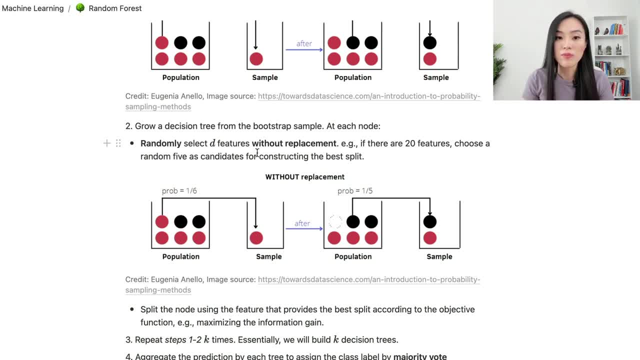 constructing the best split For a bagging algorithm. we actually consider all features of the bagging algorithm. For example, if we want to construct a bagging algorithm, we use the features to be candidates for constructing the best split. That's the only. 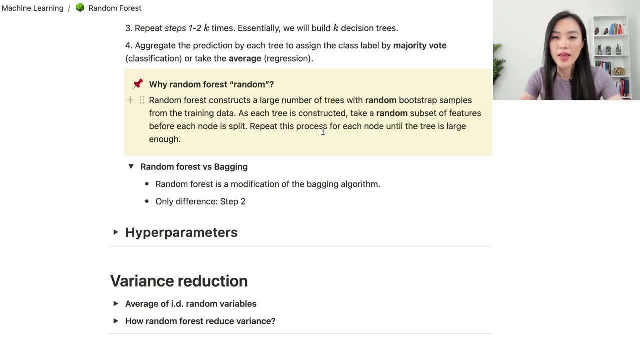 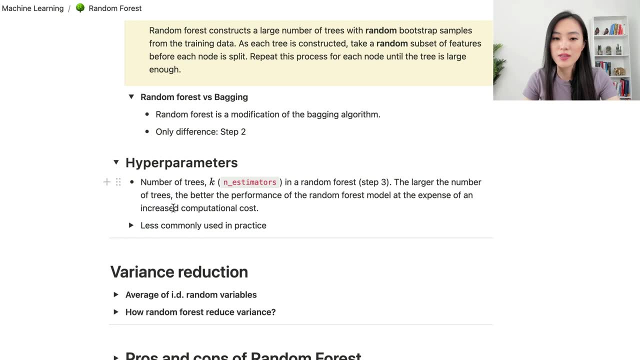 difference between random forest and bagging. Okay, now let's look at the hyperparameters involved in a random forest model. The most important hyperparameter is the number of trees k in a random forest. In step 3, we mentioned that we need to construct k decision trees. 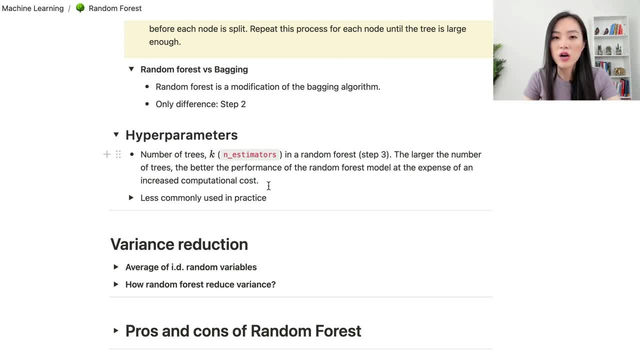 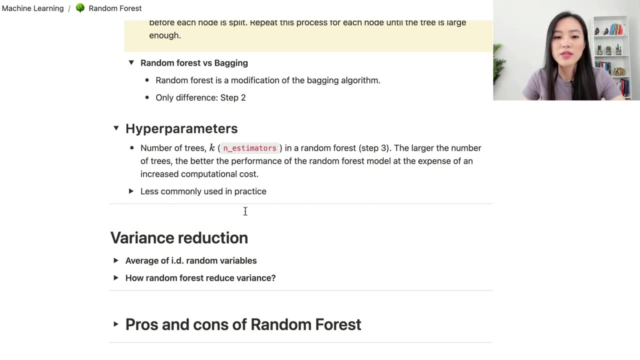 The larger the number of trees, the better the performance of the random forest model at the expense of an increased computational cost. So we want to construct many decision trees, but we also need to consider the computational cost of doing that. There are also some less commonly used hyperparameters, in practice meaning that 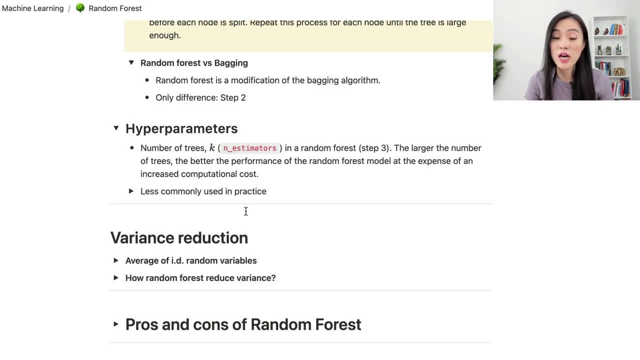 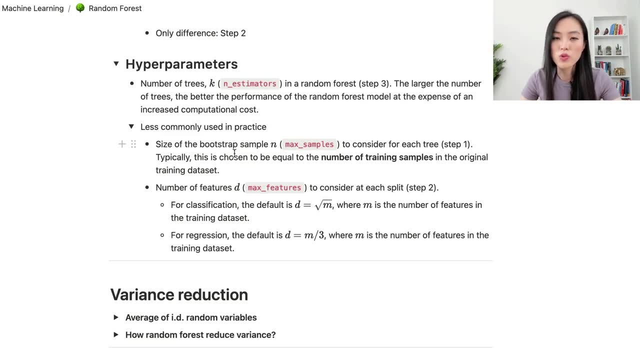 we can use some default values instead of spending lots of time and effort tuning those hyperparameters. One hyperparameter is the size of the bootstrap sample n to consider for each tree. Typically this is chosen to be equal to the number of training samples in the original training dataset. 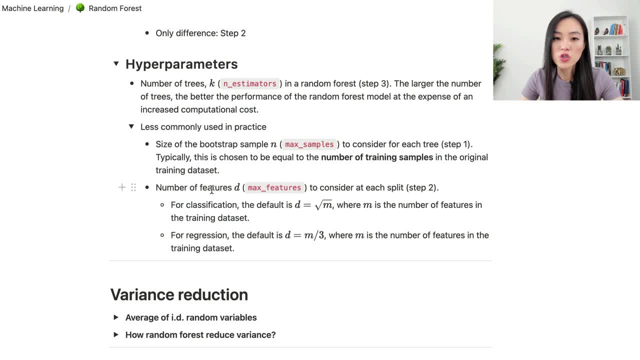 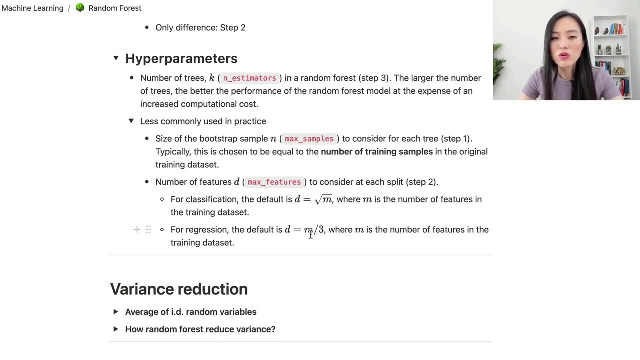 Another hyperparameter is the number of features d to consider at each split. For classification tasks, the default is: d is square root of m, where m is the number of features in the training dataset. For regression tasks we can use: d equals m over 3. Again. 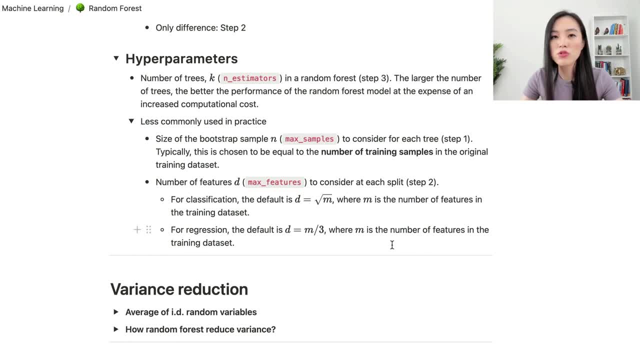 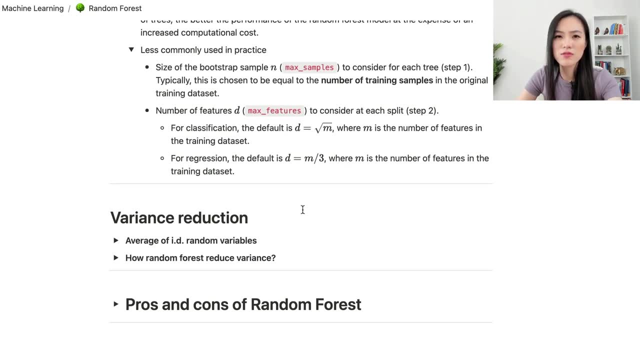 m is the number of features in the training dataset. So those are the hyperparameters for a random forest model. Next let's look at how does random forest reduce variance? This is really important to understand because there are lots of interview questions related to this topic. 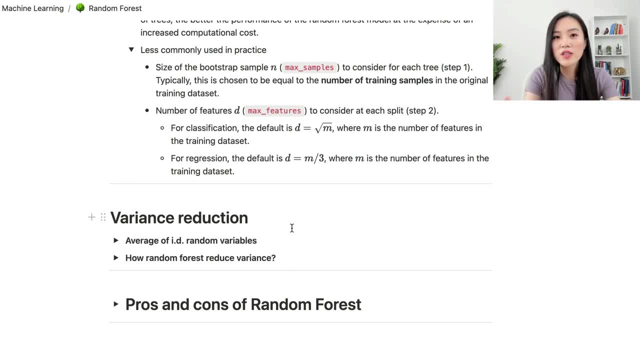 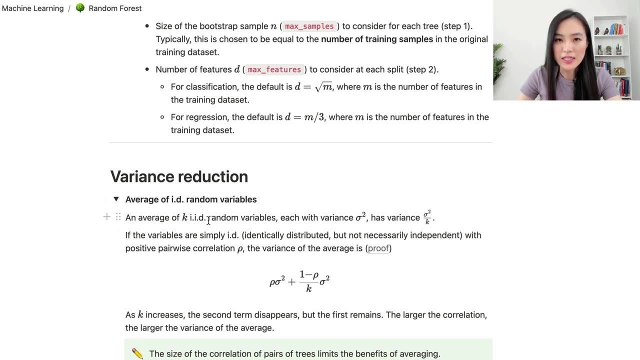 We will touch on some formulas, but don't worry, they are not hard to understand. If you can follow my logic, then it's easy for you to understand how random forest reduces variance. Okay, let's first look at the average of iid random variables. So if we have k, iid independent, 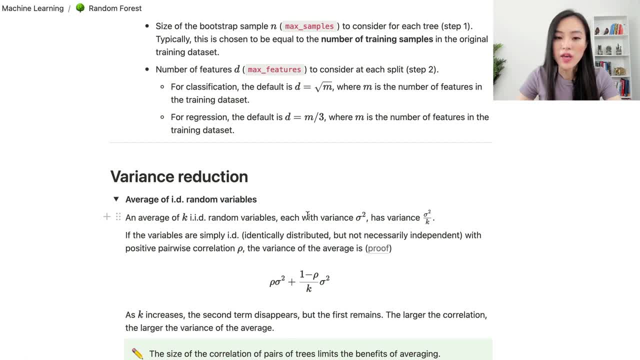 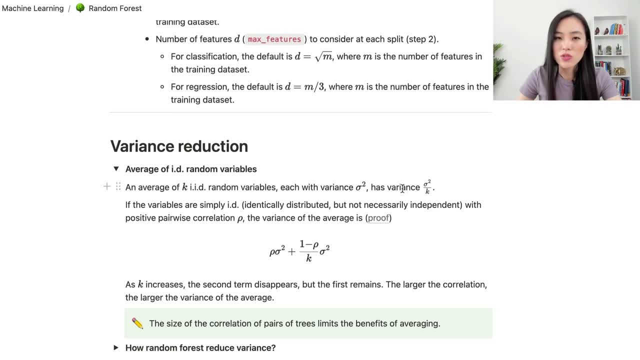 and identically distributed random variables, each with variance sigma squared. then we look at the average of them and the average should have variance sigma squared over k. Right, we know this based on the central limit theorem If the variables are simply iid. 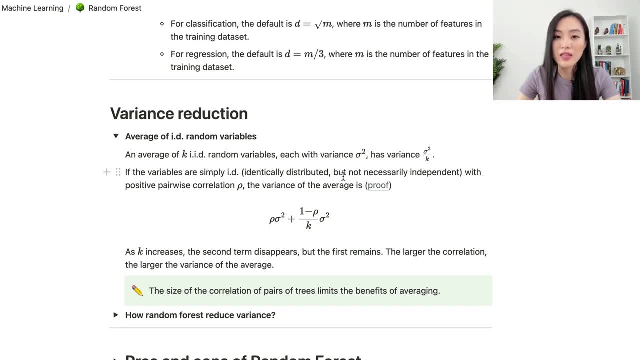 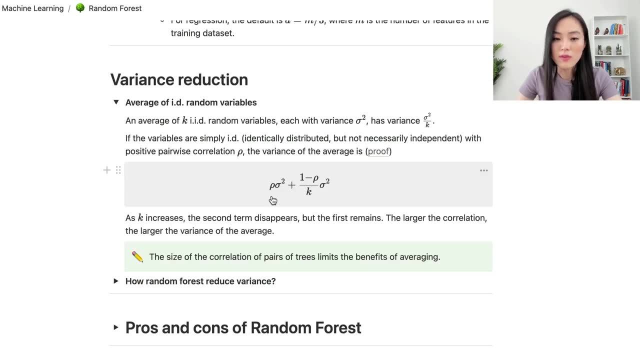 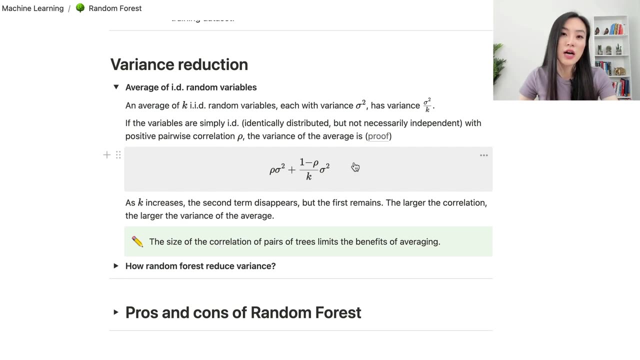 identically distributed but not necessarily independent. with the positive pairwise correlation rho. the variance of the average is: rho sigma squared plus 1, minus rho over k sigma squared. The proof of this formula is out of scope, so we will not go into the detail of this video, but if you are interested, 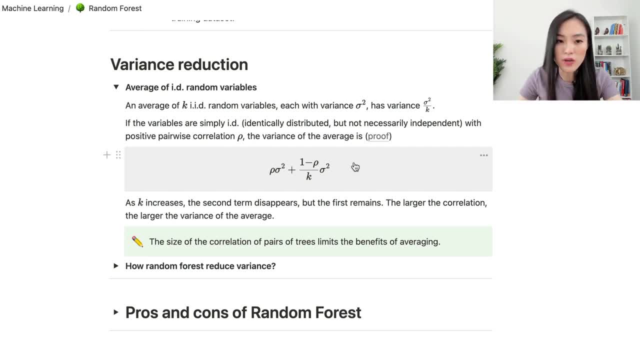 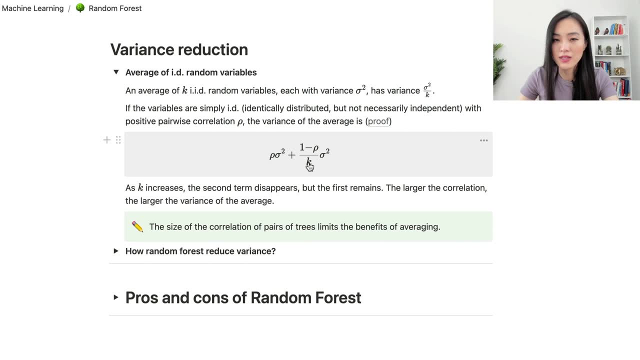 I have the link in the video description so that you can learn about the proof of this formula. So, based on this, we know that as k increases, the second term disappears, right, because k is in the denominator, but the first term remains. So it means that the larger the pairwise correlation. 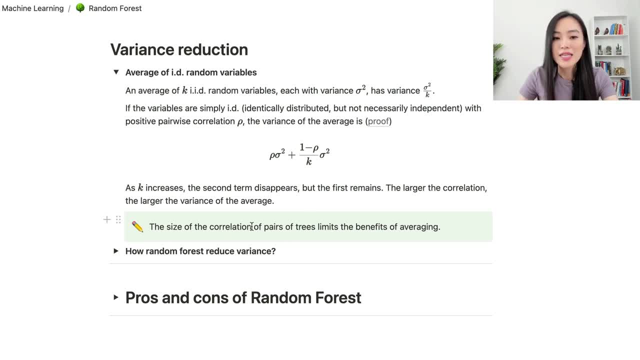 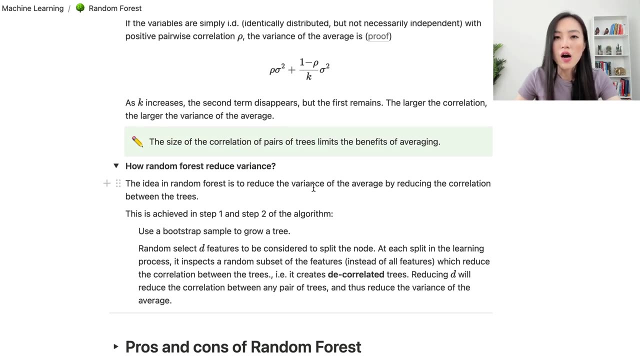 the larger the variance of the average. In the context of a random forest, it means that the size of decision trees limits the benefit of averaging. Now, in terms of how random forest reduces variance, the idea is to reduce the variance of the average by reducing the correlation between: 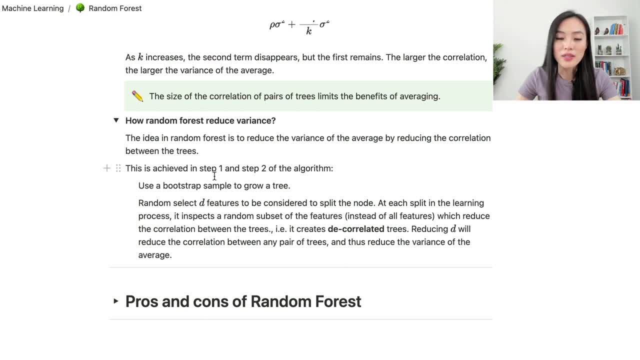 decision trees. This is achieved in step 1 and step 2 of the algorithm. In step 1, we use a bootstrap sample to grow a tree, so each tree will be built based on different bootstrap samples. In step 2, we select d features to be considered to split the tree node At each split in the learning process. 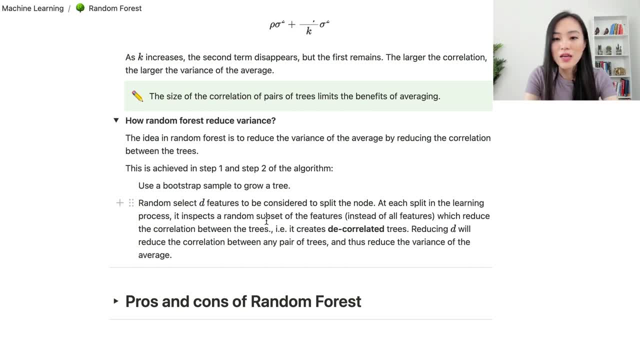 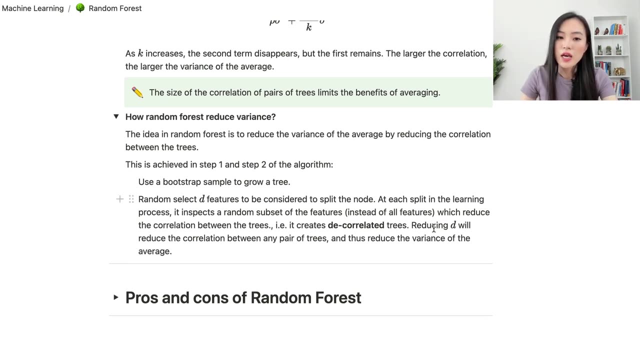 it inspects a random subset of the features, instead of all features, which reduce the correlation between the trees, meaning that it creates d-correlated trees. Creating d-correlated trees is a very important concept in random forest. If we reduce d, we reduce the correlation. 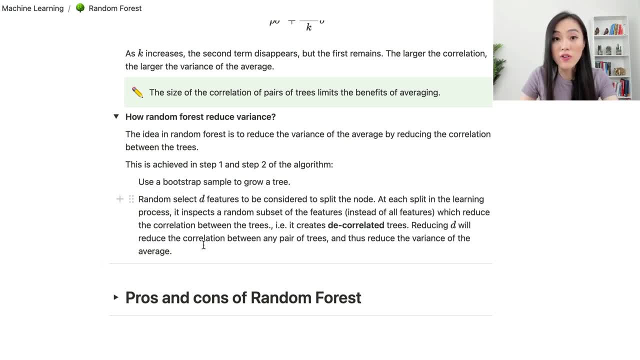 between any pair of trees and therefore reduce the variance of the average. So, in the context of a random forest, the average is d-correlated trees. So that's how random forest reduces variance by creating d-correlated decision trees. Okay, at this point you have learned all the. 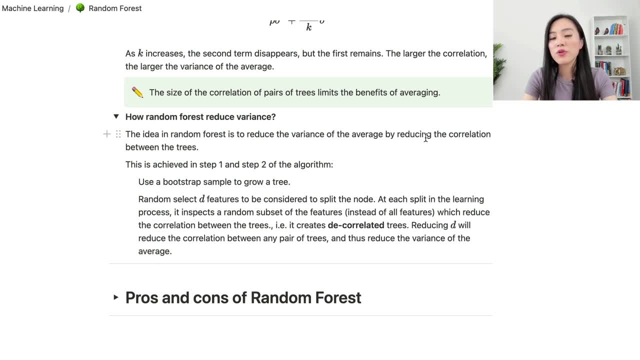 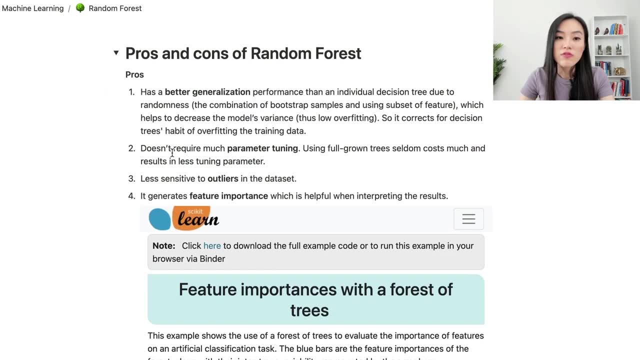 important concepts related to random forest which will help you answer interview questions. Finally, let's look at the pros and cons of random forests. First of all, a random forest has better generalization performance than individual decision trees due to randomness. We have talked about how random forests introduce randomness in the algorithm. It helps to